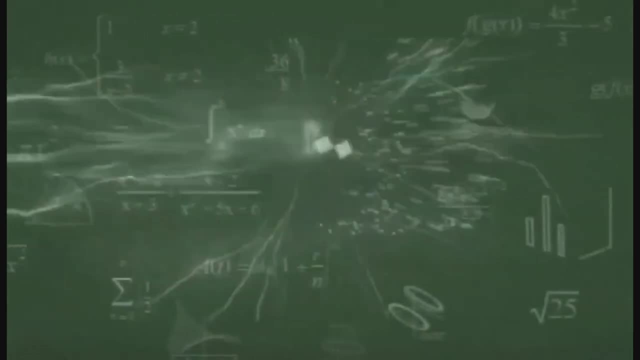 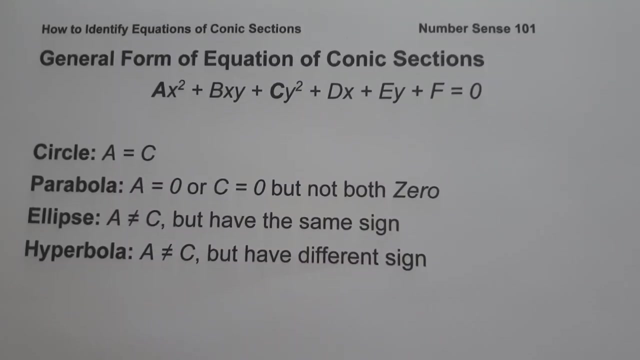 For today's video. we are going to talk about how to identify the equations of conic sections and we are going to explain everything in details. The general form of equation of conic sections is written in the form of ax square plus bxy plus cy square plus dx plus ey plus f equals zero. 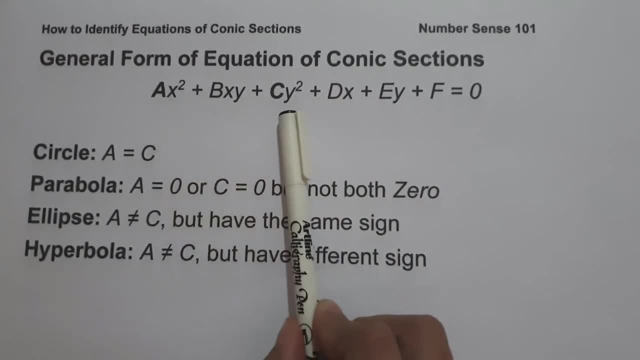 If the coefficient of x square is equal to the coefficient of y square, we can say that the given equation is a circle. And if the value of a or the value of c is equal to zero, but not both equal to zero, that means if you don't have an x square term or y square term. 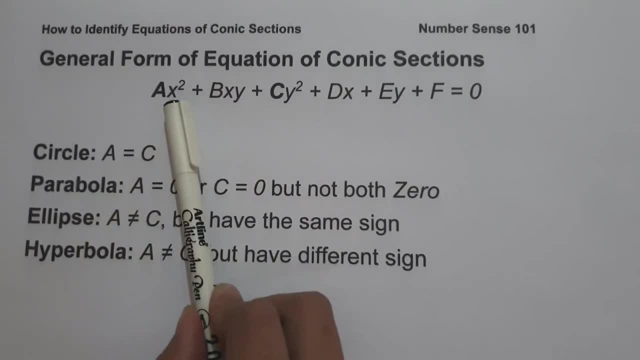 the given equation is a parabola. And if the coefficient of x square is not equal to the coefficient of y square, but they have the same sign, we can say that the given equation is an ellipse. And lastly, if the coefficient of x squared is not equal to the coefficient of y, 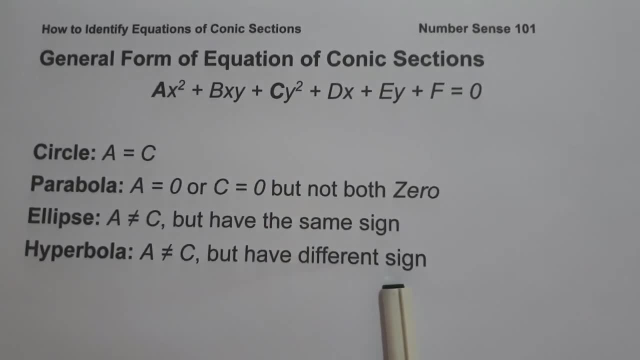 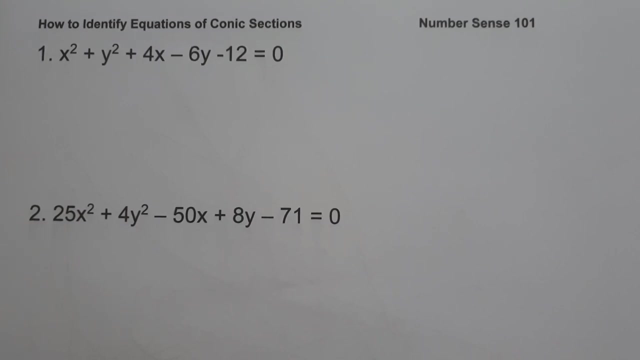 squared, but they have different sign. we can say that the given equation is a hyperbola. So these are the basic concepts that you need to remember in order for us to identify the equations of conic sections. So let's start and let's have an example. On the given set of examples we are: 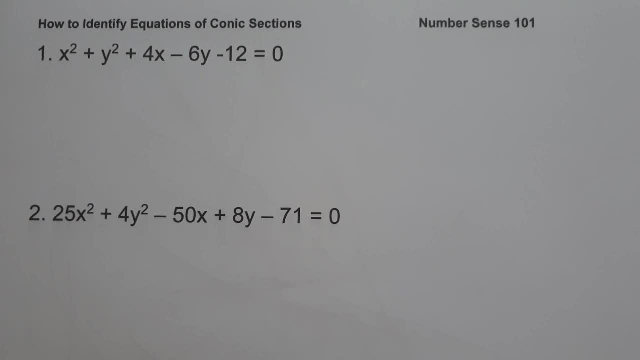 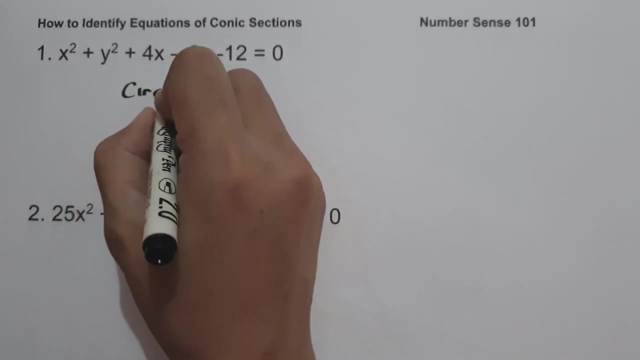 going to identify the conic sections using the given equations. On number 1,, x squared plus y squared, plus 4x minus 6y minus 12 equals 0.. Since the coefficient of x squared and y squared are the same, we can say that this equation is a circle, And this will be our answer. 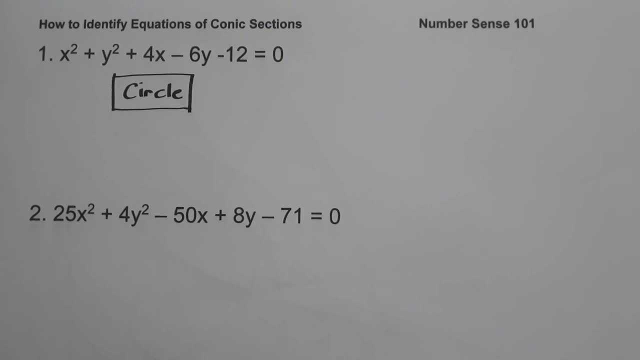 On number 2, we have 25x squared plus 4y squared, minus 50x plus 8y minus 71 equals 0.. Since the coefficient of x squared is not equal to the coefficient of y squared, but they have the same sign, therefore we can say that this equation is an ellipse. 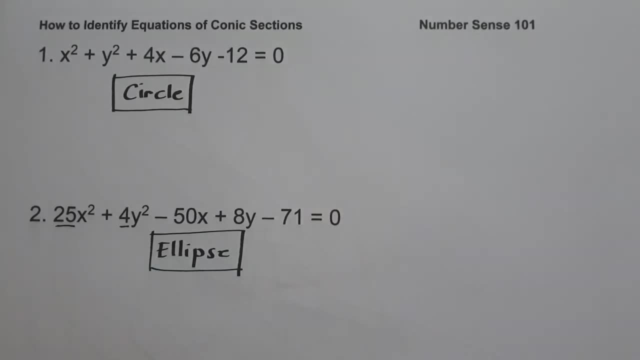 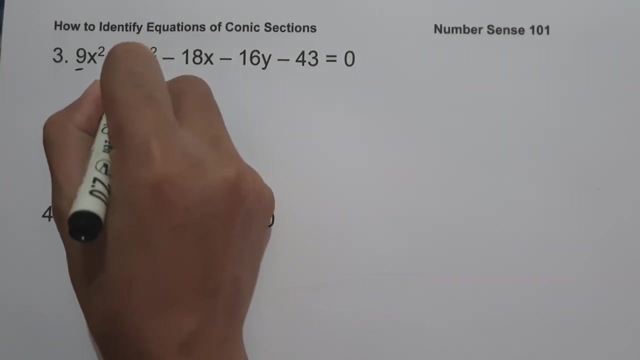 So this will be our answer. On example number 3,: 9x squared minus 4y squared minus 18x minus 16y minus 43 equals 0.. Since the coefficient of x squared is not equal to the coefficient of y squared, at the same time they don't have the same sign. 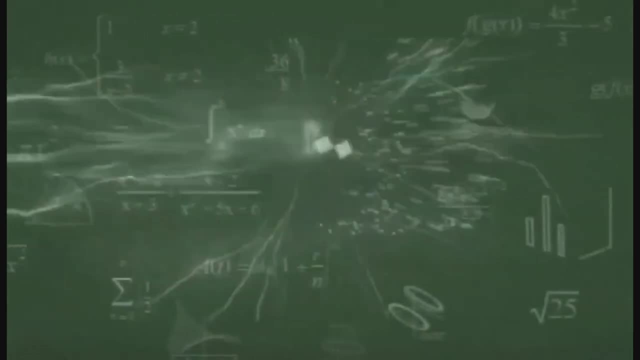 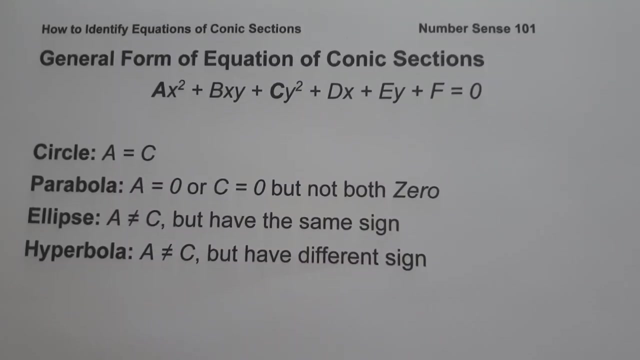 For today's video. we are going to talk about how to identify the equations of conic sections and we are going to explain everything in details. The general form of equation of conic sections is written in the form of ax square plus bxy plus cy square plus dx plus ey plus f equals zero. 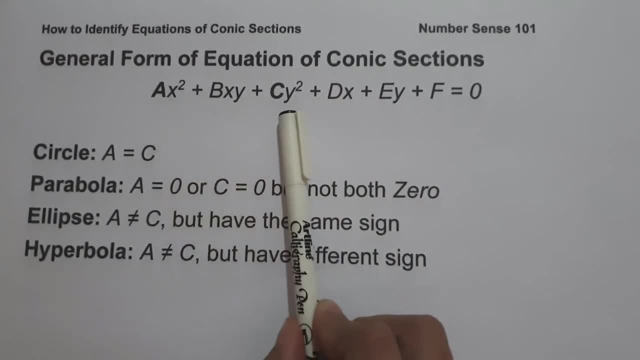 If the coefficient of x square is equal to the coefficient of y square, we can say that the given equation is a circle. And if the value of a or the value of c is equal to zero, but not both equal to zero, that means if you don't have an x square term or y square term. 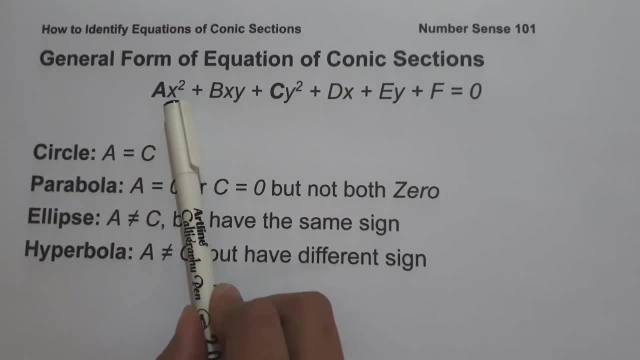 the given equation is a parabola. And if the coefficient of x square is not equal to the coefficient of y square, but they have the same sign, we can say that the given equation is an ellipse. And lastly, if the coefficient of x square is not equal to the coefficient of y, 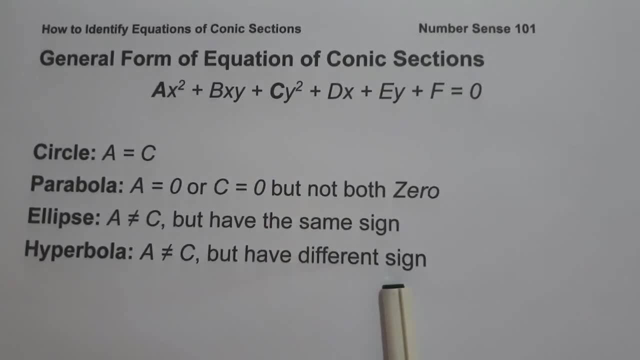 square, but they have different sign. we can say that the given equation is a hyperbola. So these are the basic concepts that you need to remember in order for us to identify the equations of conic sections. So let's start and let's have an example On the given set of 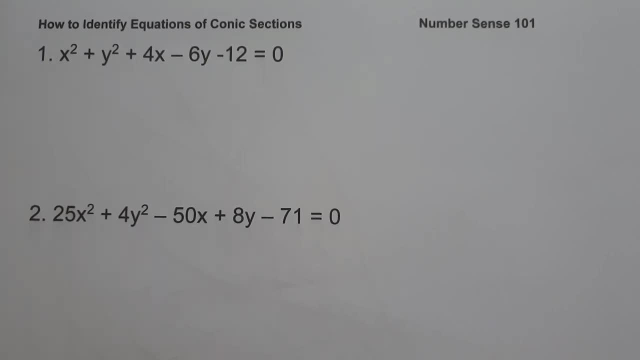 examples. we are going to identify the conic sections using the given equations On number one: x square plus y square plus 4x minus 6y minus 12 equals zero. Since the coefficient of x square and y square are the same, we can say that this equation is a circle, And this will be our answer. 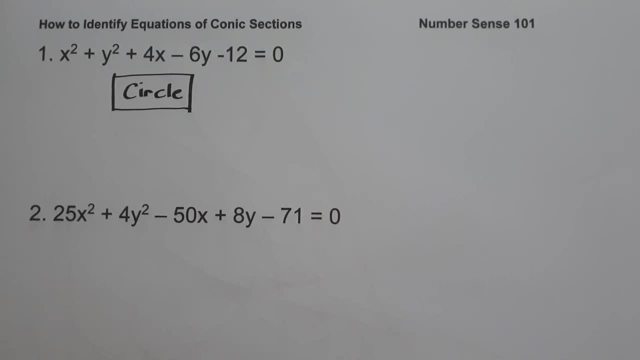 On number two, we have 25x square plus 4y square minus 50x plus 8y minus 71 equals zero, Since the coefficient of x square is not equal to the coefficient of y square, but they have the same sign. therefore, we can say that this equation is an ellipse. 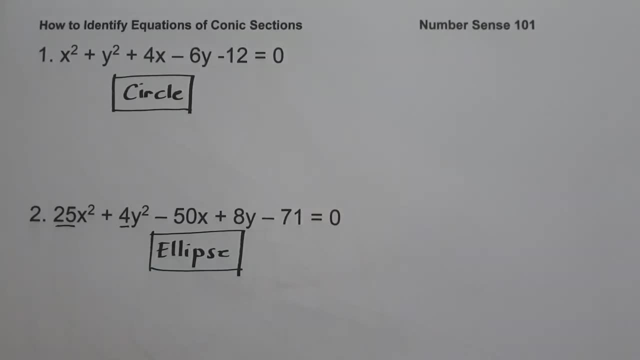 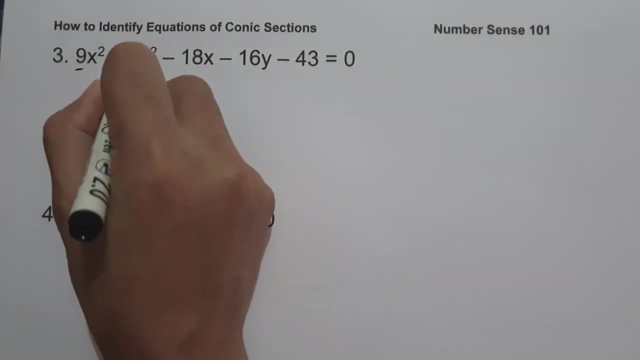 So this will be our answer On example number three: 9x square minus 4y square minus 18x minus 16y minus 43 equals zero, Since the coefficient of x square is not equal to the coefficient of y square. 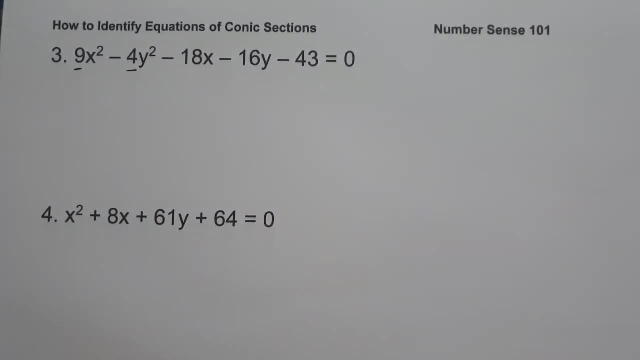 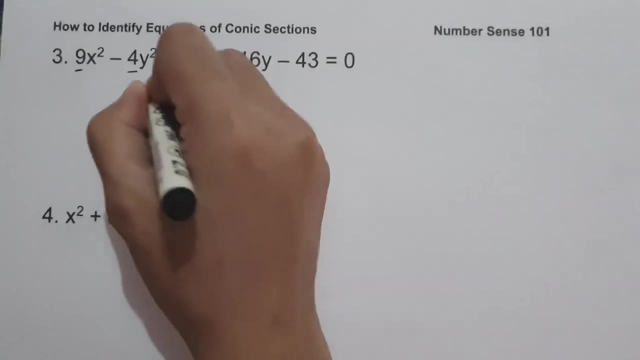 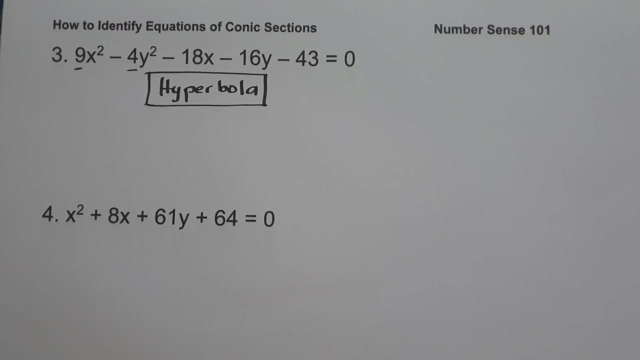 at the same time, they don't have the same sign. therefore, we can say that this equation is a hyperbola. So this will be our answer. On number four, we have x square plus 8x plus 61y plus 64 equals zero. 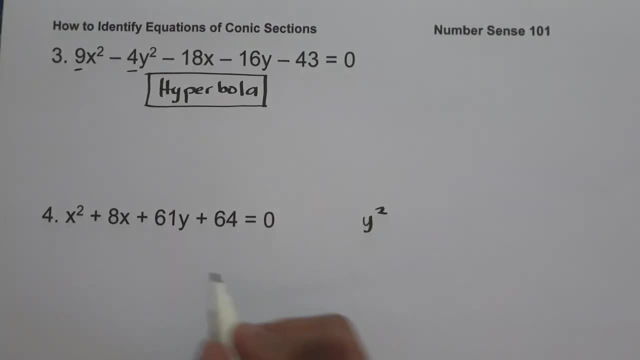 Since we don't have y square, we can say that this equation is a parabola. So this will be our answer. On example number five: 16x square plus 81y square minus 324y minus 972 equals zero. 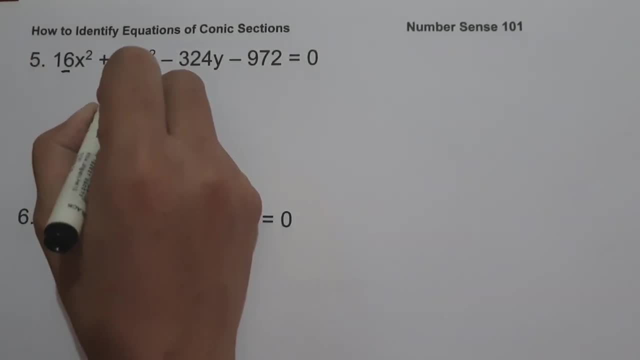 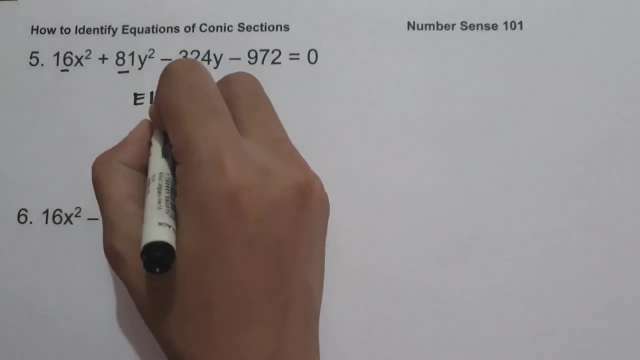 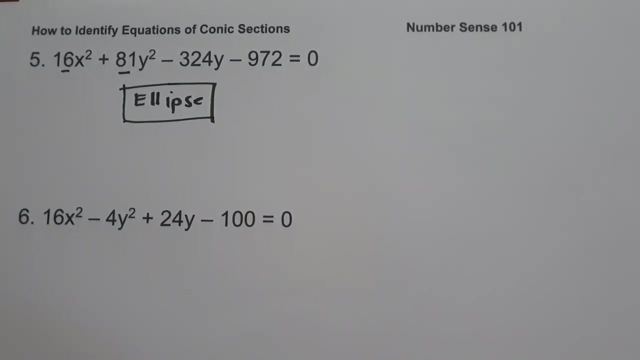 Since the coefficient of x square is not equal to the coefficient of y square, but they have the same sign, we can say that this equation is an ellipse. So this will be our answer. On number six, we have 16x square minus 4y. 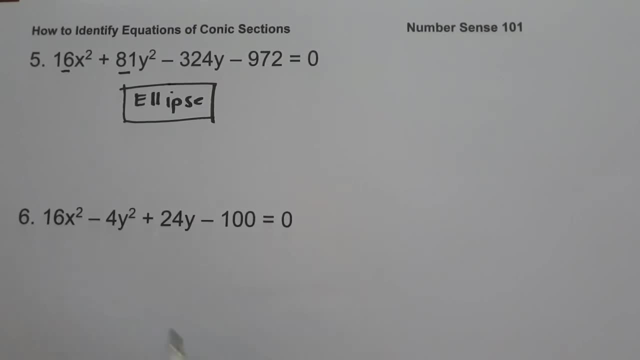 Since the coefficient of x square is not equal to the coefficient of y square, at the same time they have different sign. we can say that this equation is a hyperbola. So this will be our answer. On example number seven, we have y square minus 8x plus 10y plus 57 equals zero. 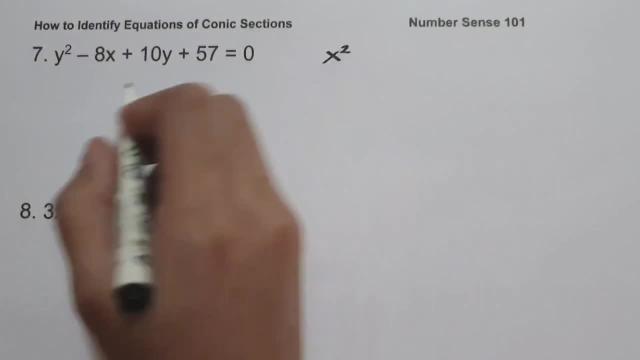 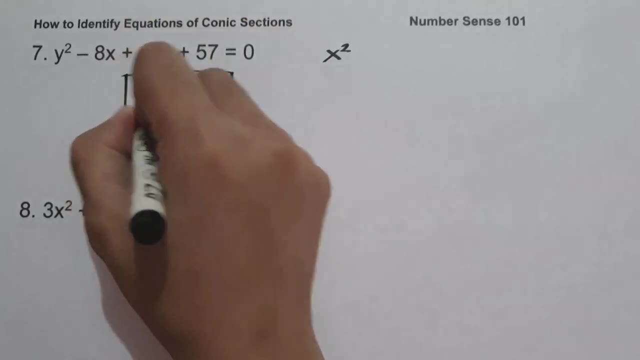 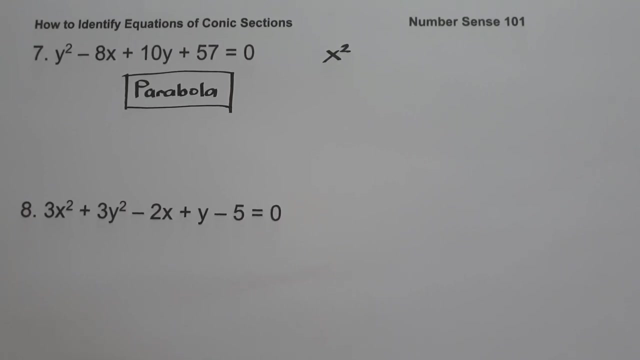 Since we don't have 8x plus 10y plus 57 equals zero, we can say that this equation is an ellipse. Since we don't have x square, we can say that this equation is a parabola. On number eight, we have 3x square plus 3y square minus 2x plus y minus 5 equals zero. 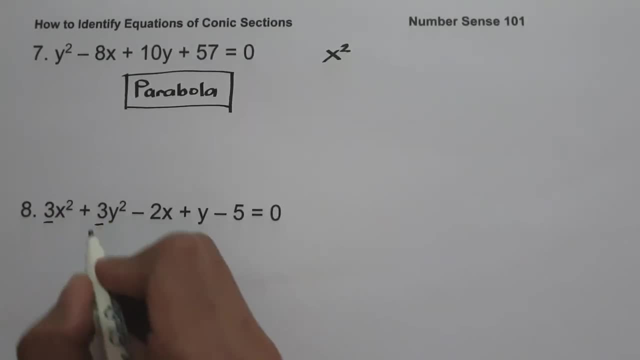 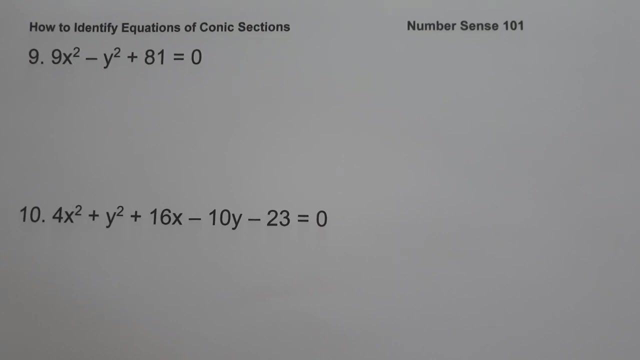 Since the coefficient of x square is equal to the coefficient of y square, we can say that this equation is a circle, And this will be our answer. On example number nine. we have 9x square minus y square plus 81 equals zero. 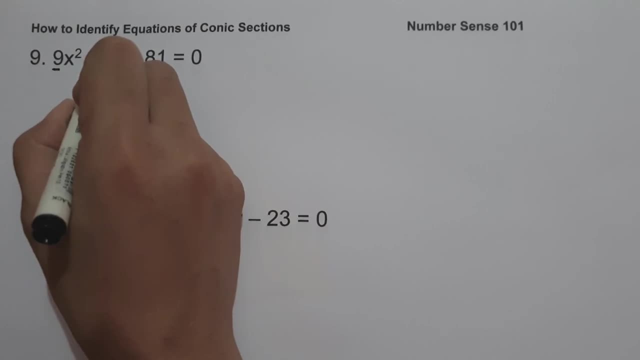 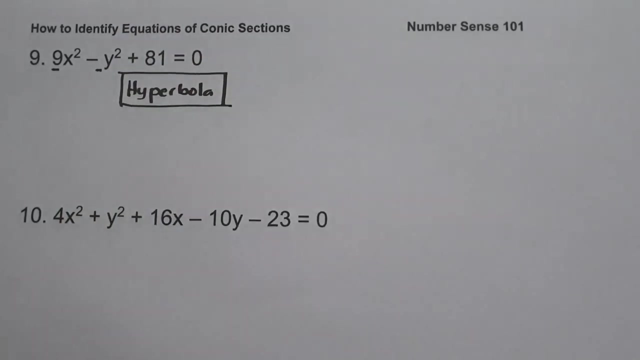 Since the coefficient of x square is not equal to the coefficient of y square, at the same time, they have different sign. we can say that this equation is a hyperbola And this will be our answer. On our last example, we have: 4x square plus y square plus 81 equals zero. 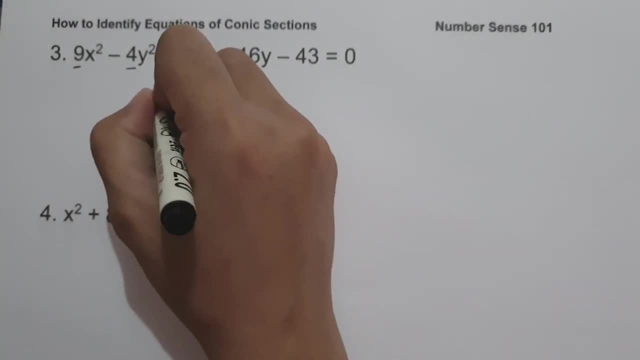 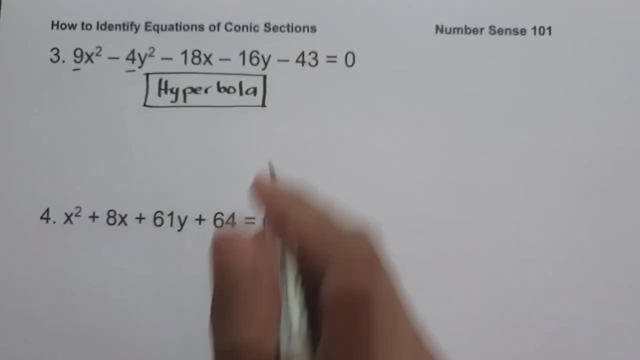 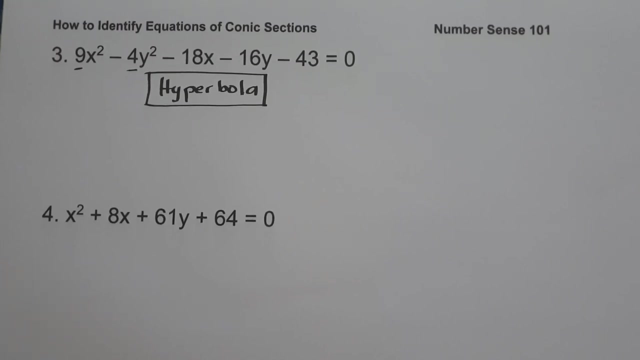 therefore, we can say that this equation is a hyperbola. So this will be our answer. On number 4, we have x squared plus 8x plus 61y plus 64 equals 0.. Since we don't have y squared, we can say that this equation is a parabola. 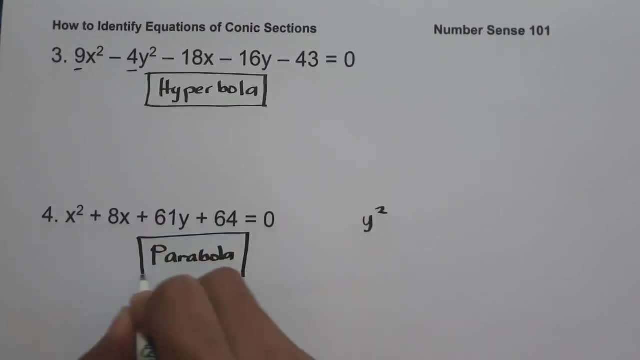 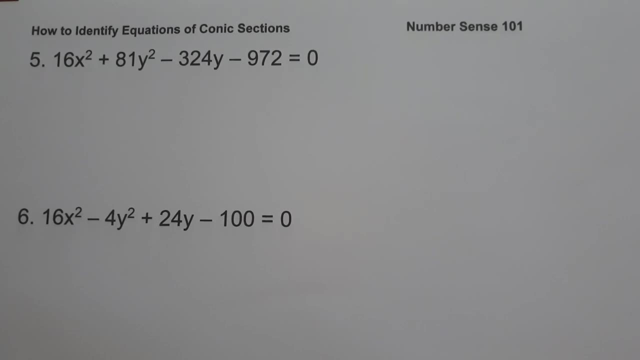 So this will be our answer On example number 5, 16x squared plus 81y squared minus 324y minus 972 equals 0.. Since the coefficient of x squared is not equal to the coefficient of y squared. but they have 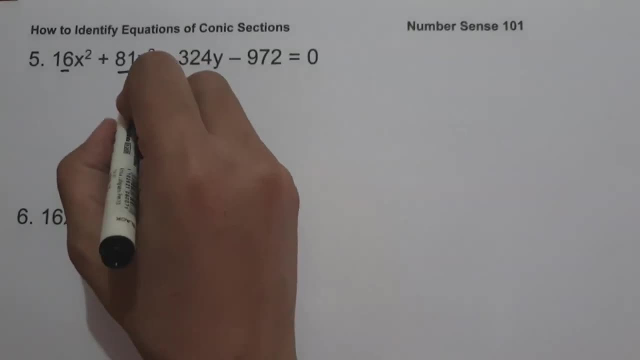 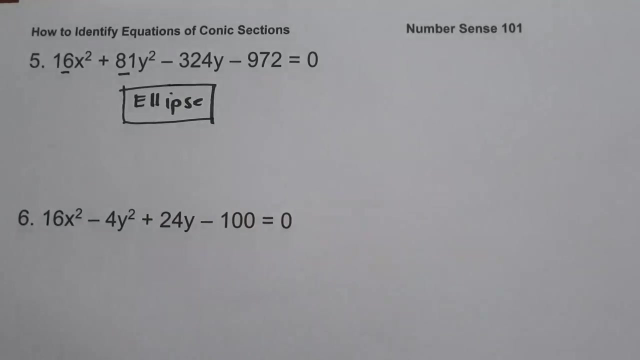 the same sign. we can say that this equation is an ellipse. So this will be our answer. On example number 6, we have: 16x squared minus 4y. squared plus 24y minus 100 equals 0.. Since the coefficient of x squared is not equal to the coefficient of y squared at the same time, 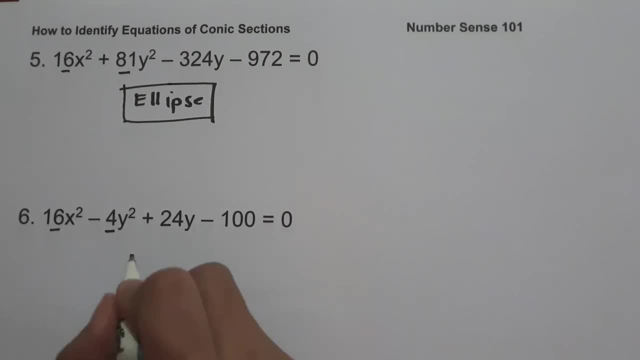 they have different sign. we can say that this equation is a hyperbola, So this will be our answer. On example number 7, we have: y squared minus 4y. squared plus 24y minus 100 equals 0.. On example number 7, we have: y squared minus 4y. squared plus 24y minus 100 equals 0.. Since the coefficient of x squared is not equal to the coefficient of y squared. at the same time, they have different sign, we can say that this equation is an ellipse. Since the coefficient of x squared is not equal to the coefficient of y squared. at the same time, they have different sign, we can say that this equation is an ellipse. Since the coefficient of x squared is not equal to the coefficient of y squared. at the same time, they have different sign, we can say that this equation is an ellipse. Since the coefficient of x squared is not equal to the coefficient of y squared. at the same time, they have different sign, we can say that this equation is an ellipse. 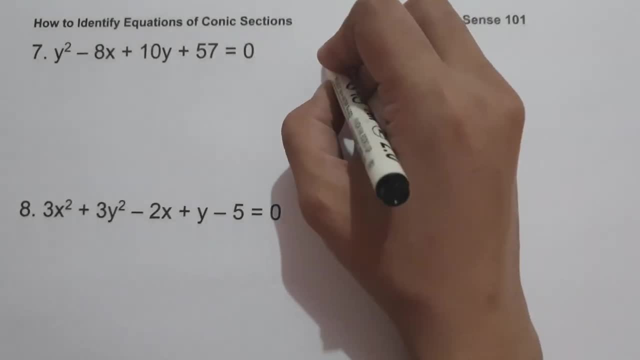 Since the coefficient of x squared is not equal to the coefficient of y squared, at the same time they have different sign. we can say that this equation is an ellipse to: 7 equals 0.. Since we don't have x square, we can say that this equation is a parabola. 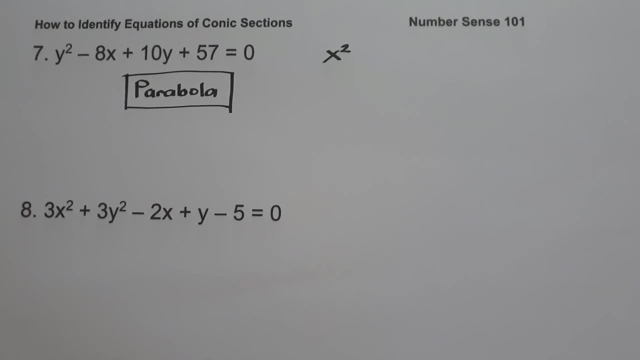 On number 8, we have 3x square plus 3y square minus 2x plus y minus 5 equals 0.. Since the coefficient of x square is equal to the coefficient of y square, we can say that this equation is a.